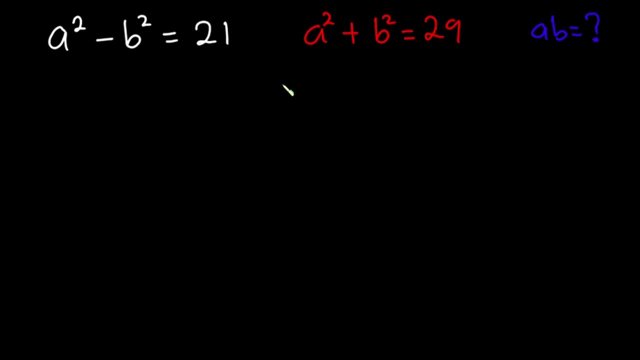 and try this first. Done Cool, Now let's get started. First we're gonna call this equation equation 1 and then call this equation equation 2.. Then from here we can say equation 1 plus equation 2.. Now, considering the left hand side of equation 1, we have a to the second power minus b. 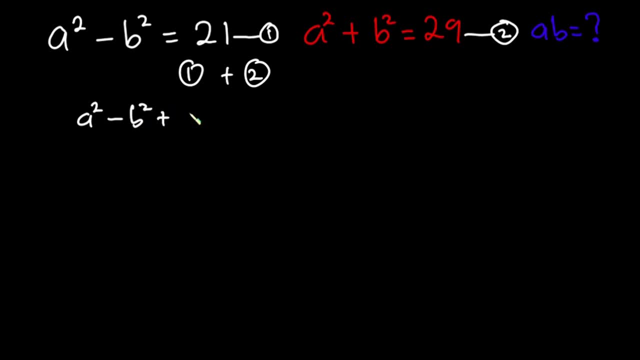 to the second power. Then from the left hand side of equation 2, we have a to the second power plus b to the second power and this is equal to 21 plus 29.. And straight away we can see that the equation 2 is equal to a to the second power minus b to the second power, is equal to 21 plus. 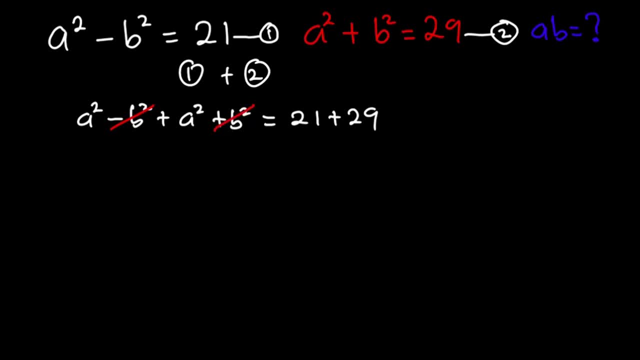 this negative b squared will cancel this positive b squared. so we have a squared plus a squared, which is 2 a squared, and this is equal to 21 plus 29, that is 50.. Since we are looking for a, let's divide inside of the equation by 2, so that this and this will go, and now we have a squared is. 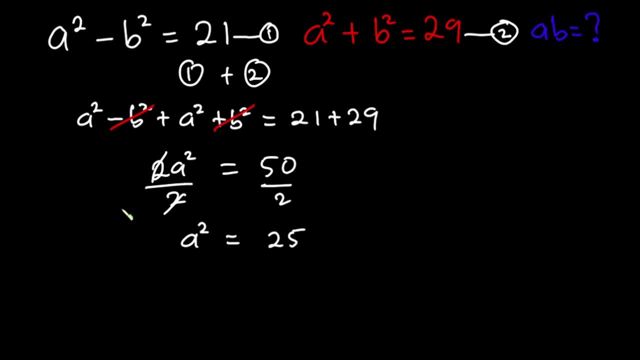 equal to 25.. Now let's go ahead and then take square root on the both side of the equation. but don't forget, we have plus or minus here. Now this square will cancel the square root. so we have: a is equal to plus or minus 5.. So now that we know the values of a, we can go ahead and then find the. 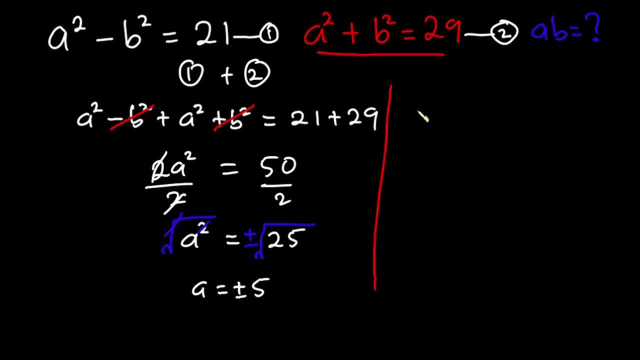 values of b from this second equation. So from this equation we can say that b squared is equal to 29.. minus a squared, b squared is equal to 29 minus. we have a to be plus or minus 5, so we're gonna have plus or minus 5 all squared, So b squared is equal to 29 minus. in other words, we'll get: 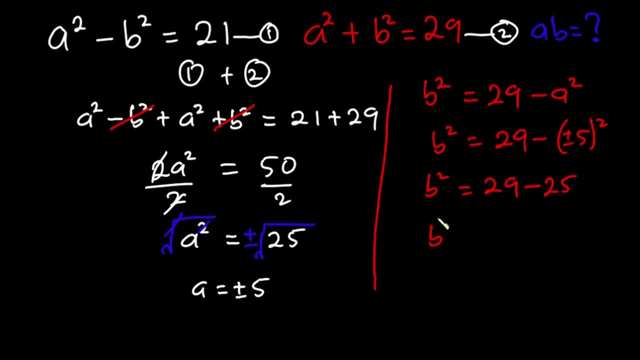 25.. So this implies that b squared is equal to 4.. Now we are looking for b, so let's take square root on the both side of the equation. Don't forget: we have plus or minus here, And straight away we can see that b squared will.